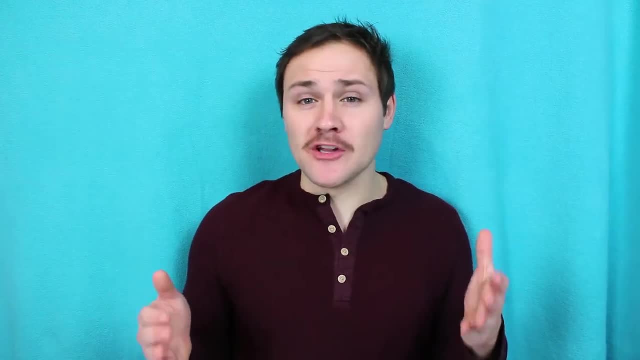 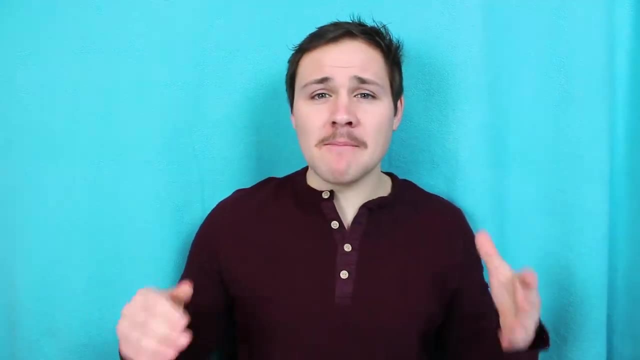 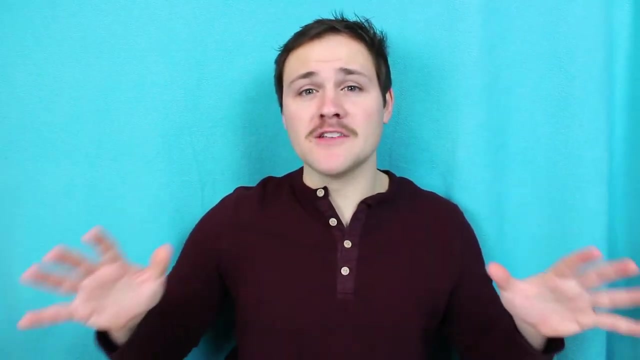 So when I set out to learn every country, I decided I was going to practice at noon on Wednesday for half an hour every week. Whatever it ends up being, pick a day or time or days or times that work for you consistently. These should be times when you have nothing else scheduled except. 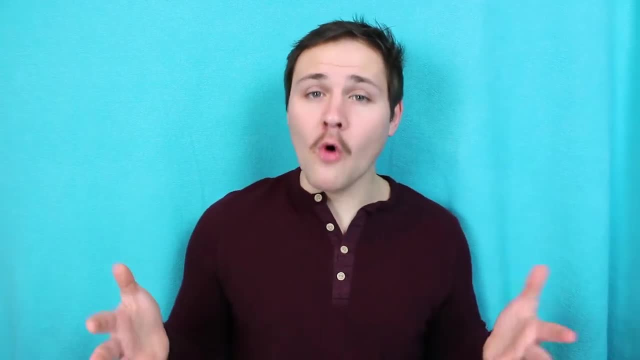 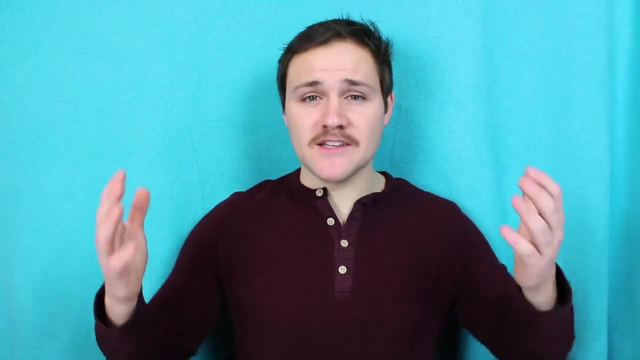 for your practice. I would suggest picking a day and time when you are always available and usually not tired. If you keep a calendar, I would block it out on your calendar And if you miss a practice, you have to make it up. So again, I wasn't in a rush to learn every country, which is why I only 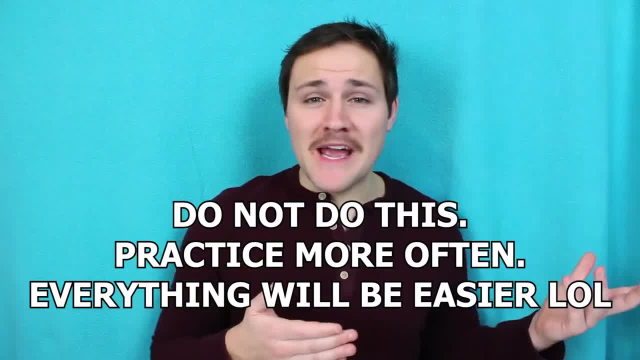 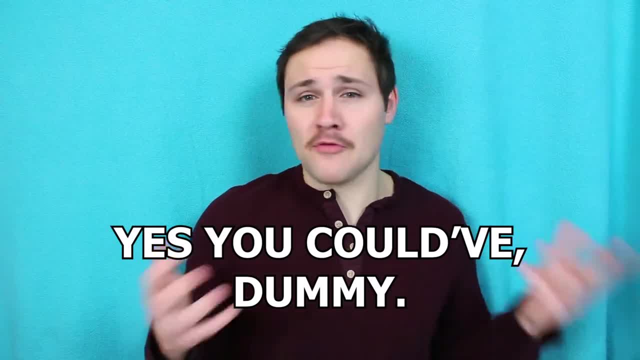 practiced once a week for about half an hour or so. At this pace, it took me three to four months to learn them all. In hindsight, I think I could have learned them much more easily if I were to practice them three days a week, so I would recommend you do something like that, But whatever. 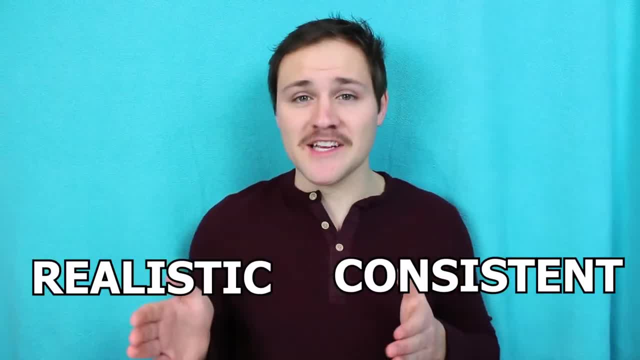 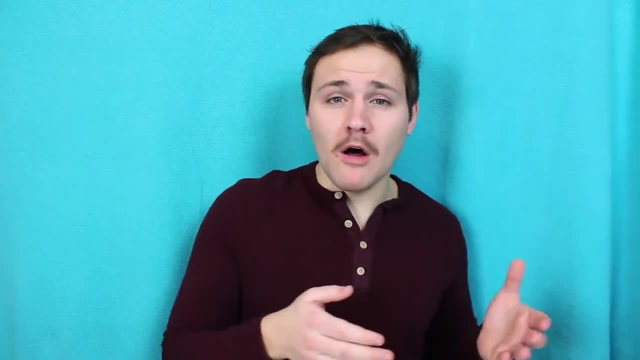 you choose to do, make sure that it is consistent and realistic. If you say you're going to practice every single day for four hours, that's probably not going to happen. I would say: start small and get in the habit of practicing, maybe increase the frequency. And I just want to say again: 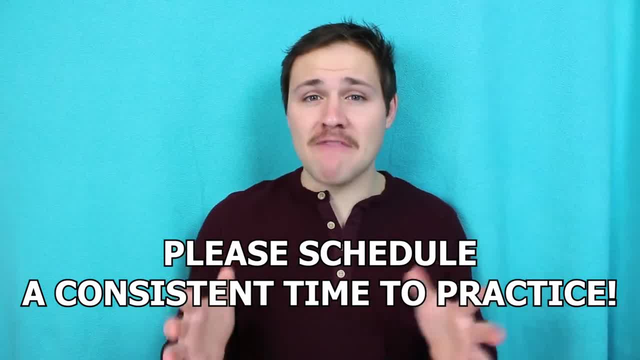 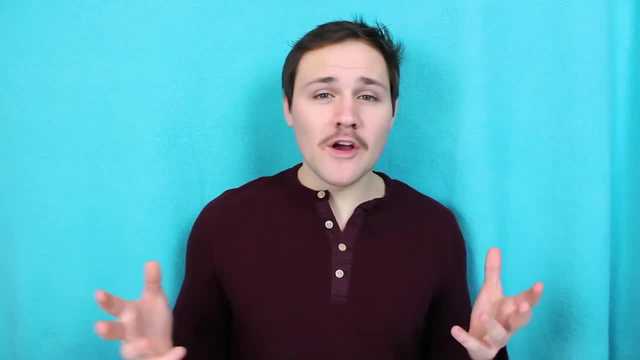 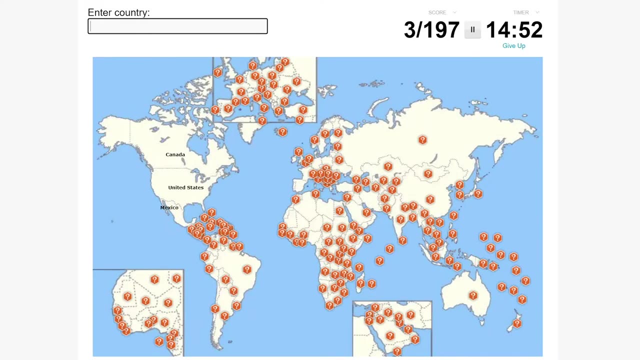 I think this is the most important part of not just learning every country, but of learning any skill and building any habit. Now we're going to get into how I actually learned every country. I started by taking the countries of the world quiz on Sporkle. once I named every country I could, so I had a baseline number that. 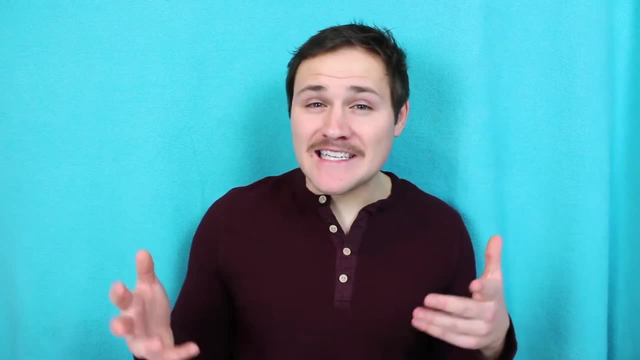 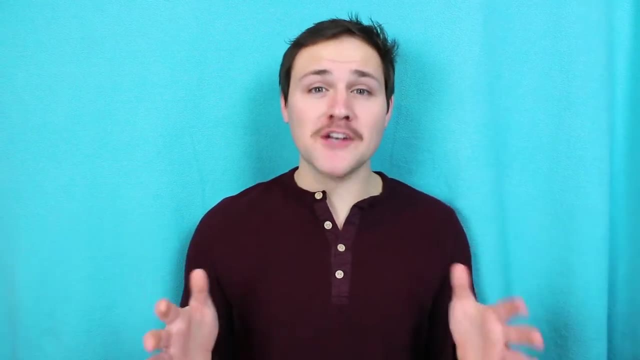 I was starting from. I don't remember what it was like. I think maybe it was like 19 or 20 countries. It was not good considering there are 197 countries Now. learning every country at once would be very, very difficult, But fortunately Sporkle has quizzes that break the world up into. 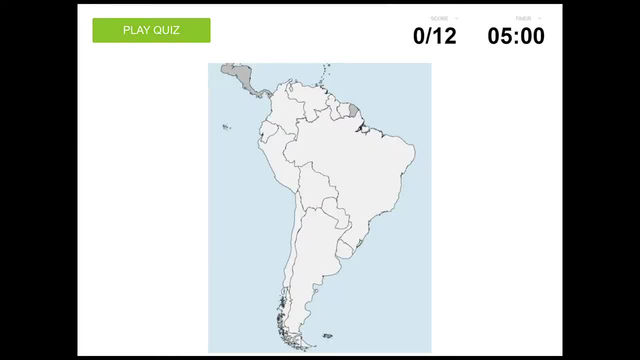 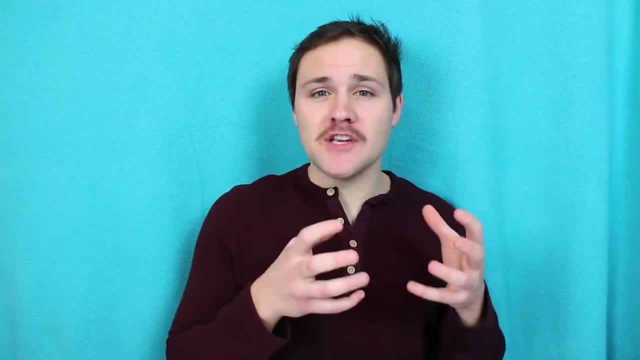 six different regions: North America, South America, Africa, Europe, Asia and Oceania. These regional quizzes divide the world into chunks that are much easier to learn, So these are what I use. I started by learning all 23 countries of North America, but I would suggest 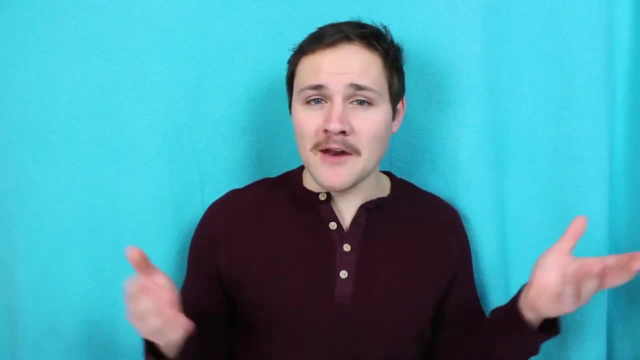 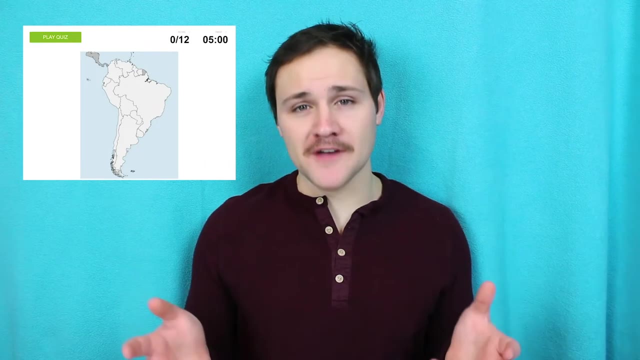 learning the countries near you, since you're probably more familiar with them and it'll make things easier. But if you do want to start in the easiest way possible, South America is the easiest region, with only 12 countries, Once you decide which region you want to start with, 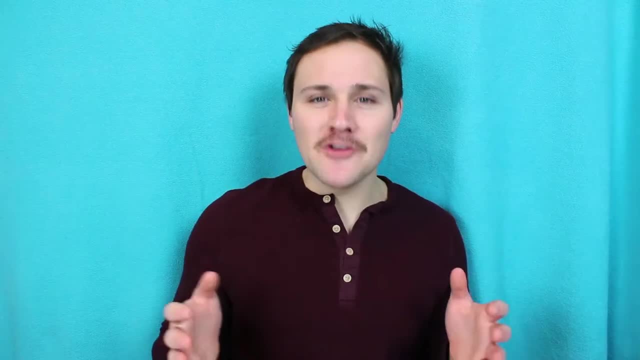 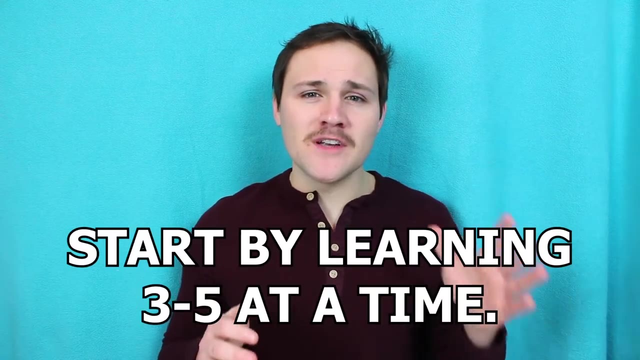 you just take the quiz over and over again. Take the quiz, see how many countries you get right and then, out of all the countries you missed, pick three to five of them to focus on learning for the next time you take the quiz, For example, in North America. I knew Canada. Mexico. but that was about it. So I took the quiz and saw that the next three countries below Mexico were El Salvador, Guatemala and Belize. So I focused on learning those three countries for the next time I took the quiz. Then, once I could remember- Canada, the US, Mexico, Guatemala. 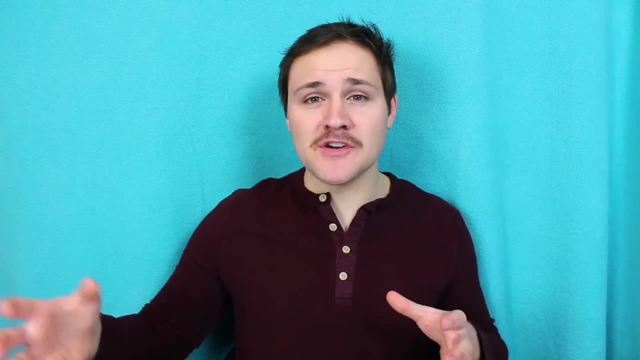 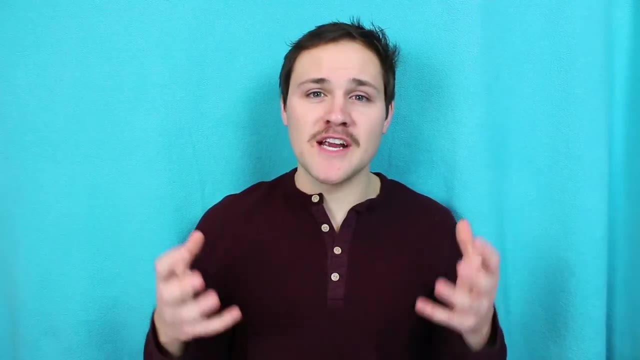 El Salvador and Belize all together. I picked another chunk of countries and focused on learning them From there. you just repeat this process over and over again until you've learned every country in the region. Now this is where learning countries takes some time, So I'm going to take a. 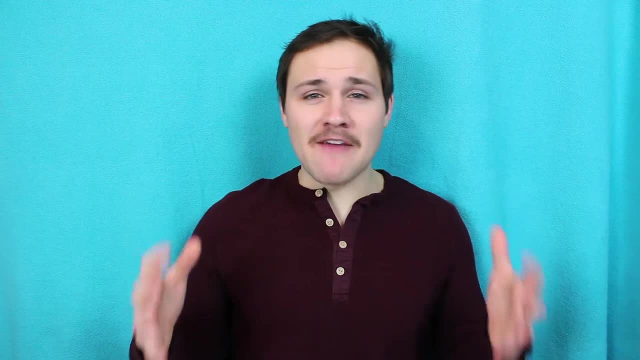 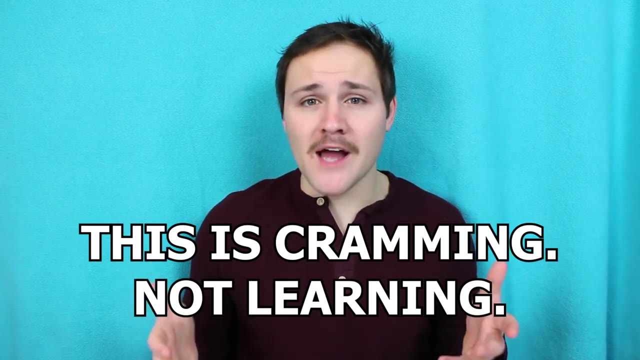 little bit of time. You have to space your learning out. If you retake the quiz every 10 minutes, you might make a lot of progress that day, but when you go to take the quiz again in another few days you probably won't remember much. That's why I recommend practicing consistently either two or 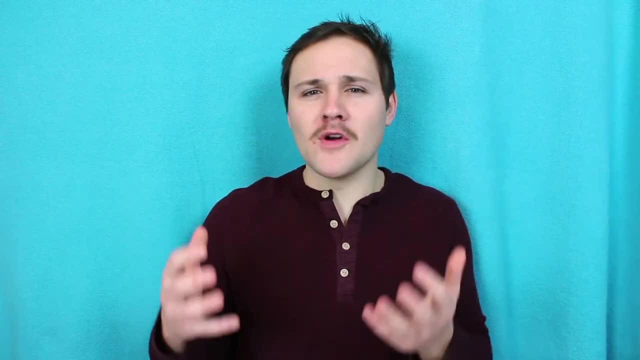 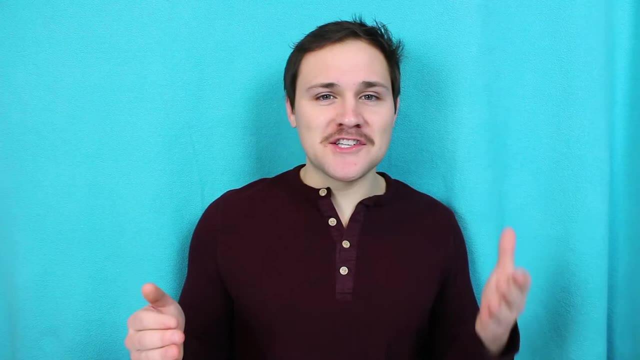 three days a week. Now, I know a lot of you are probably thinking: okay, when you say you focus on learning the countries, what are you actually doing? Well, this is where you're going to have to find learning tricks that work for you. One way to do this is through associations, For example. 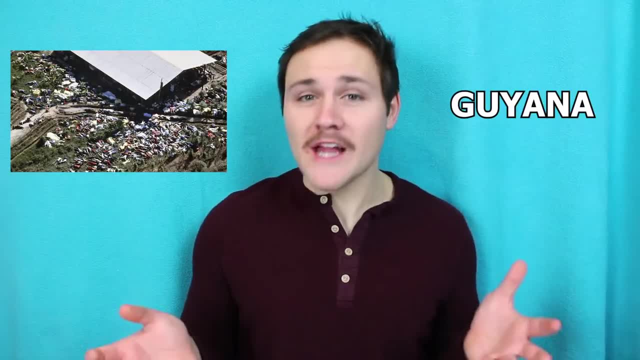 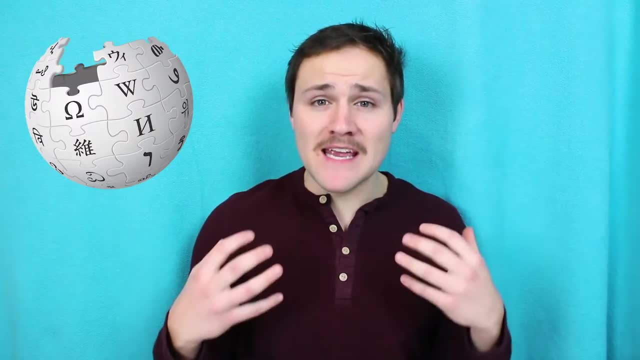 I associated Guyana with the cult of Americans that drank poisoned Kool-Aid there, And if I didn't know anything about the country, I would skim their Wikipedia page until something stuck out to me, and then I would focus on memorizing that as a way to learn every country, For example. 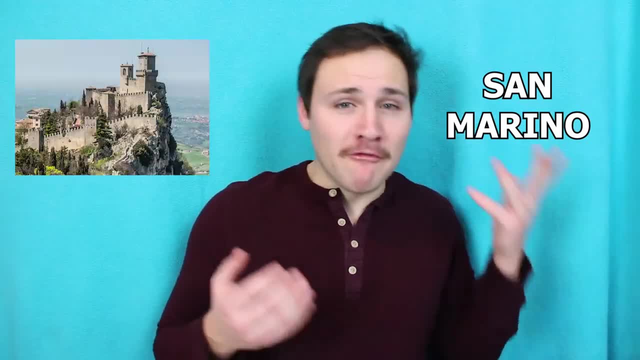 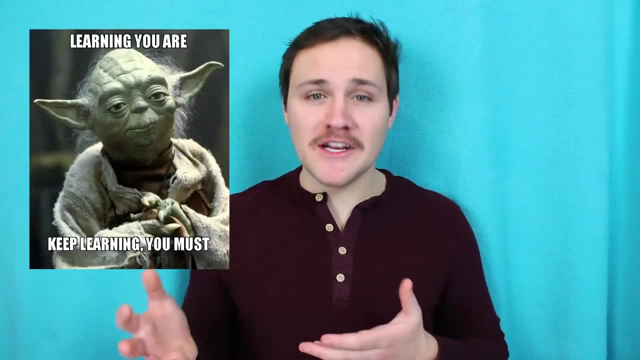 I didn't know anything about San Marino, but then I learned that they're basically a fortress nation on a mountain and that helped me remember the country. This makes it easier to remember countries and you're actually learning something about them, which is pretty cool, In my opinion. 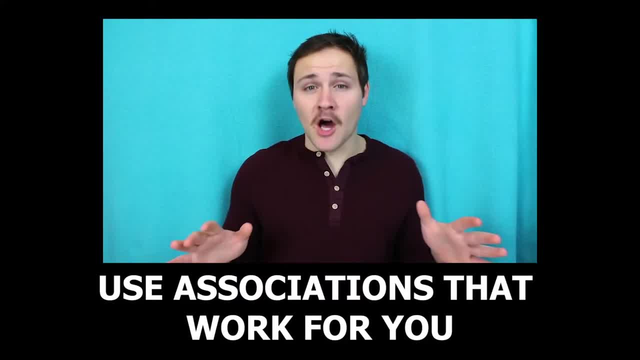 it's totally okay to associate a country with a country that you don't know about, but if you're familiar with the country, it's okay to associate a country with something that's completely unrelated to it, if it helps you remember the country. For example, I remembered the country. 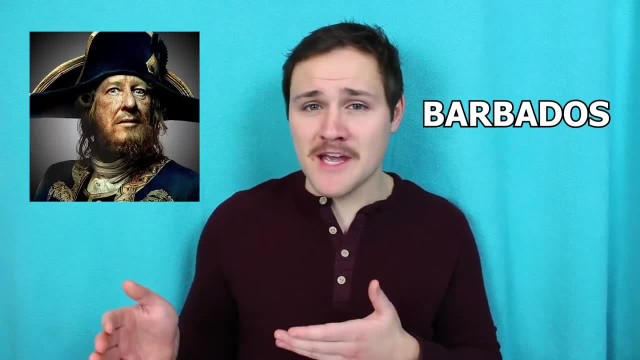 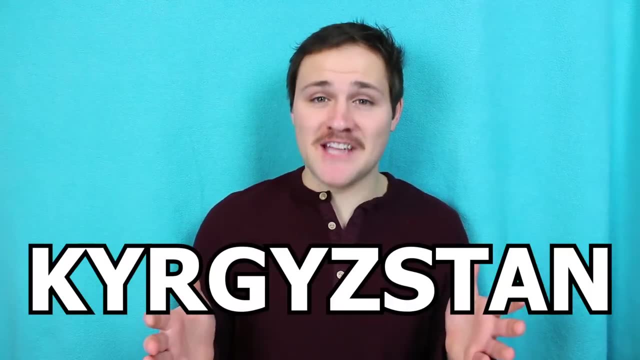 Barbados by thinking of Barbossa from Pirates of the Caribbean. Those things are completely unrelated but they helped me remember the countries. Sometimes you'll have trouble spelling a country like Kyrgyzstan. It took me so long to spell this country. In these cases. 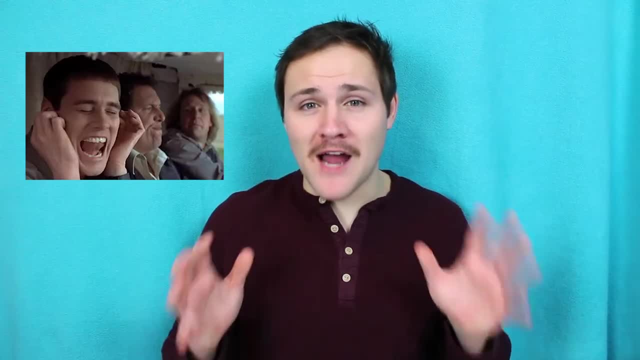 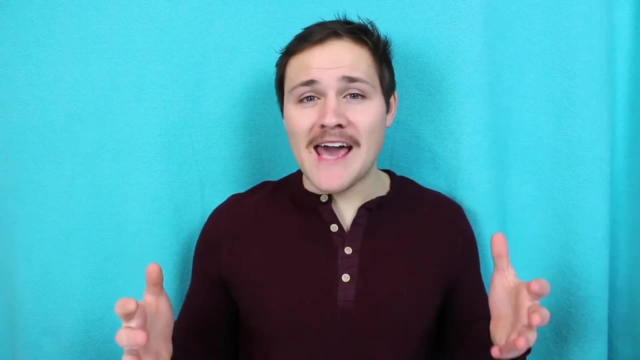 what I did was completely ignore the correct way the country was pronounced and instead made up a way that they were pronounced in my head. that would help me remember how to spell them. For example, in my head I didn't pronounce it Kyrgyzstan, I pronounced it Kyrgyzstan. 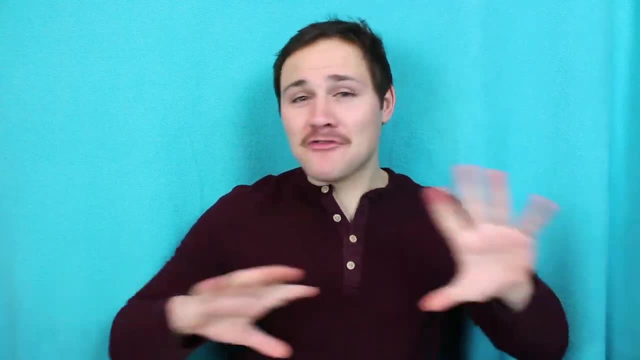 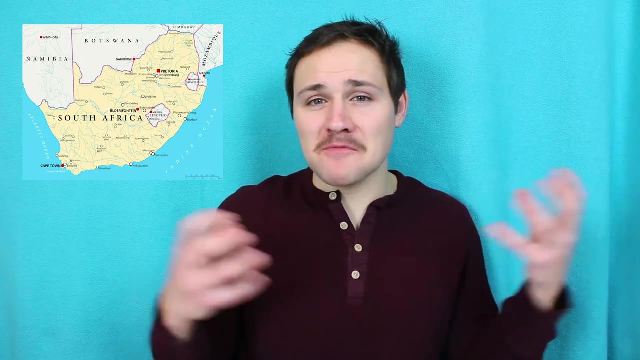 because that's the way it was spelled and that's what helped me remember it. Then, after I had memorized all the countries, I was able to go back and remember it as Kyrgyzstan. Sometimes it can be easier to learn countries together as opposed to individually. At the end, 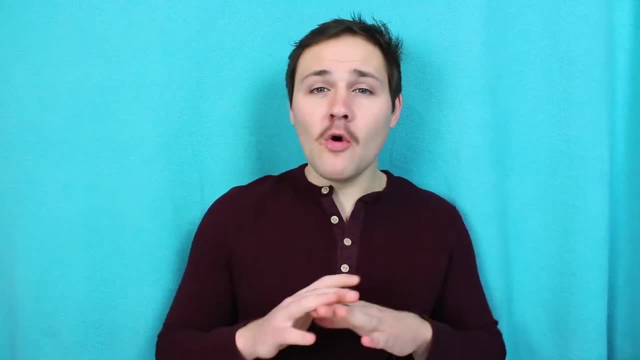 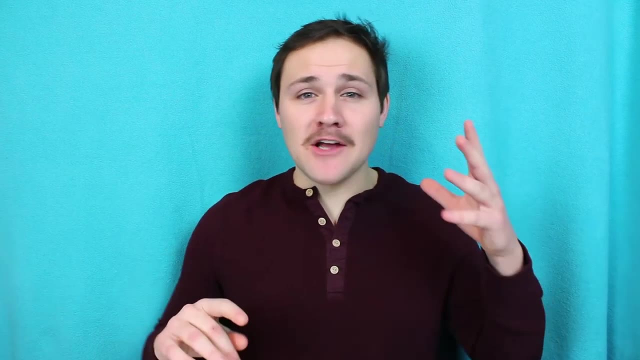 of the day, you have to develop learning hacks that work for you. There is no good trick or bad trick in my book. If it works, it works. You can always go back after you've learned everything and erase all the bad associations or stereotypes or little tricks, and then you can go back and 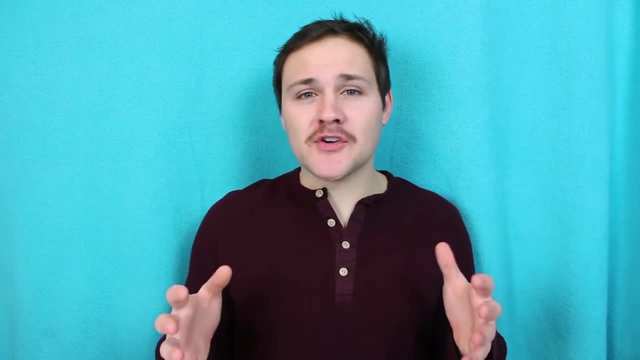 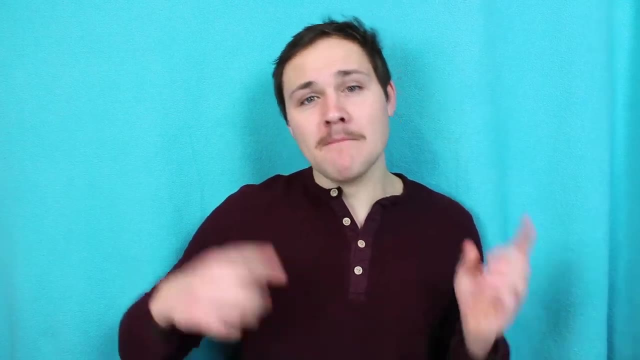 remember a country, You'll know you've learned every country in a region. when you're able to pass the quiz every time, you take it with considerable ease. Once you've gotten to that point, you can move on to a quiz for another region. Now here's the important part. Once 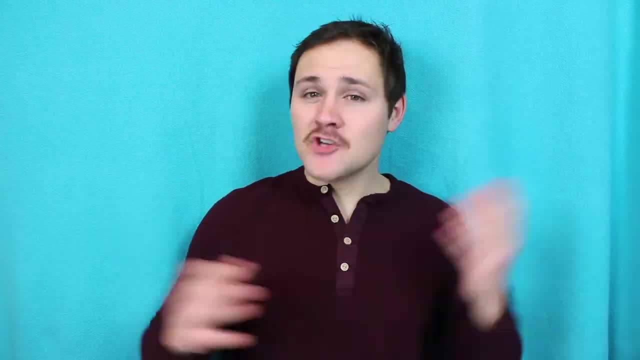 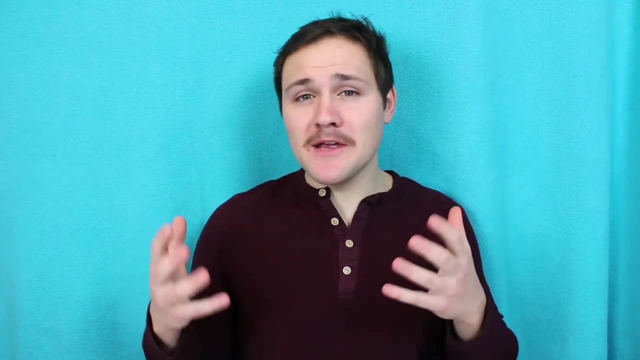 you've learned every country in a region. keep practicing them. Just because you know every country in North America doesn't mean when you start learning Europe you should not test yourself on North America. This is extremely important for keeping all of the countries in your long-term. 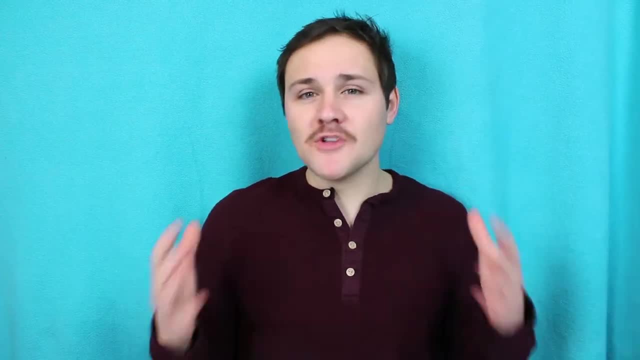 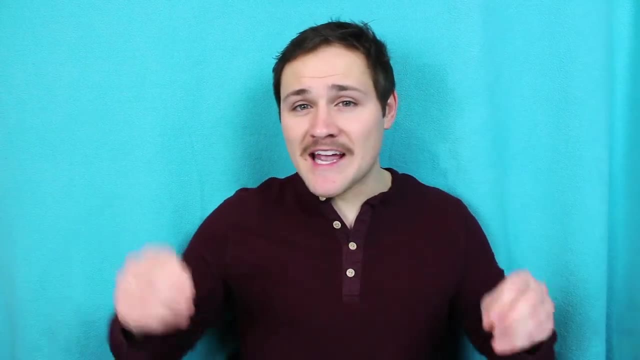 memory, which is what you're going to need to have when you take the final exam. Once you get more comfortable learning the countries, you can start to study multiple regions at once, but be aware that if you do this too early, it can really jumble stuff in your head. 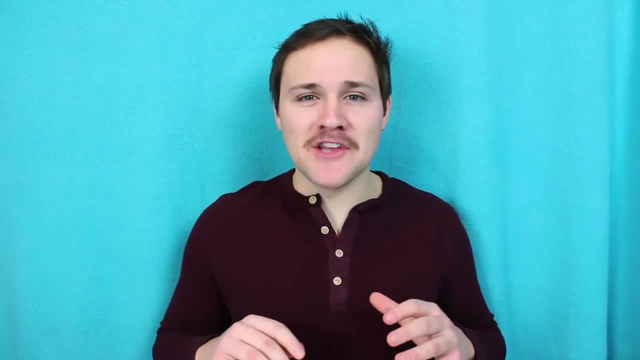 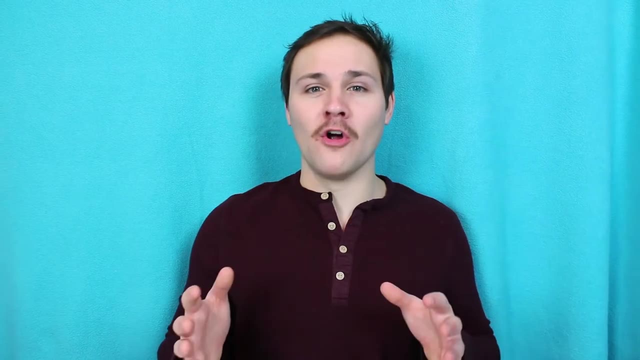 and make it harder to learn them. at the end of the day, Eventually, you'll get the hang of things, though, and this process of learning countries will become very easy Once you've mastered naming every country in every region of the world. it's time to move on to the final test. 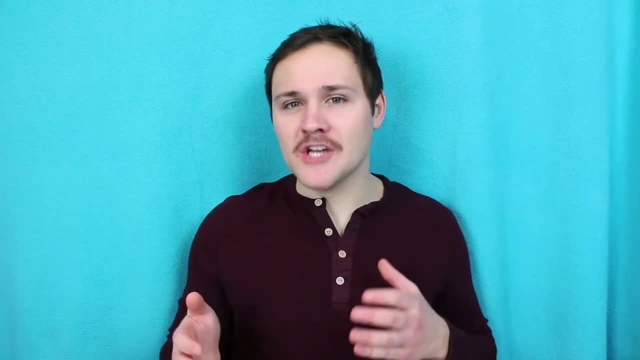 Eventually, you should be able to name every country in every region without much difficulty. If you're not good at it, you should be able to name every country in every region without much difficulty. If there are a few countries you're still stuck on, focus only on. 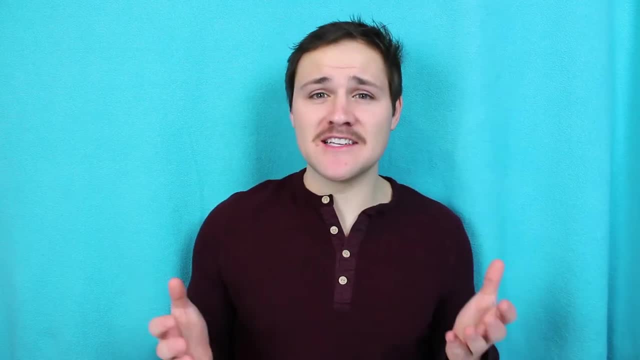 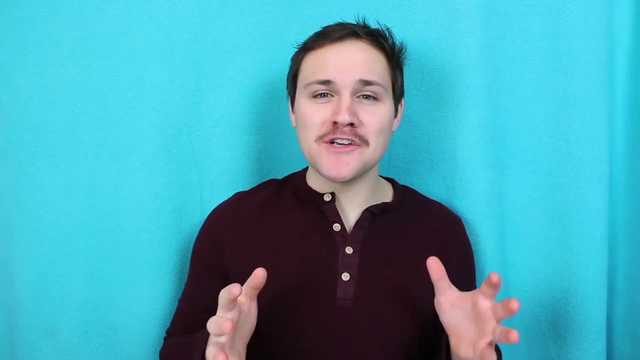 them for a few practice sessions until you can remember them just as easily as all the other countries. Yes, I'm talking about you, Timor-Leste and Brunei. At this point, you can take the countries of the world quiz. When you first start this quiz and the timer starts ticking. 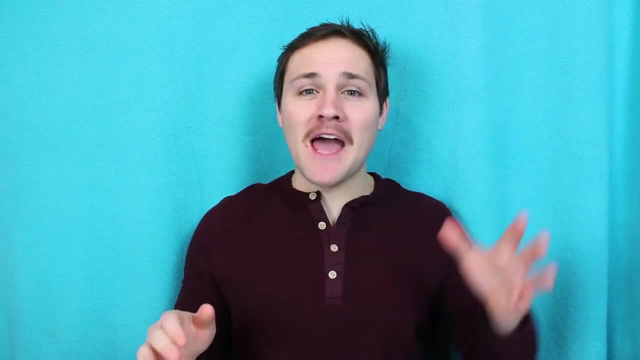 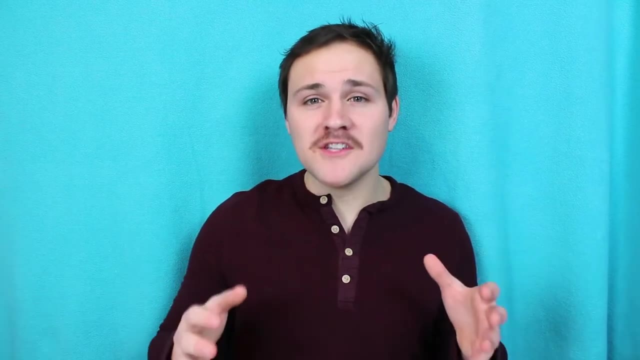 it can be very overwhelming, But take a breath, take your time and go through the world region by region. If you miss a country or two in a region, keep going and come back to them once you've finished. If you're not good at it, you should be able to name every country in every region. 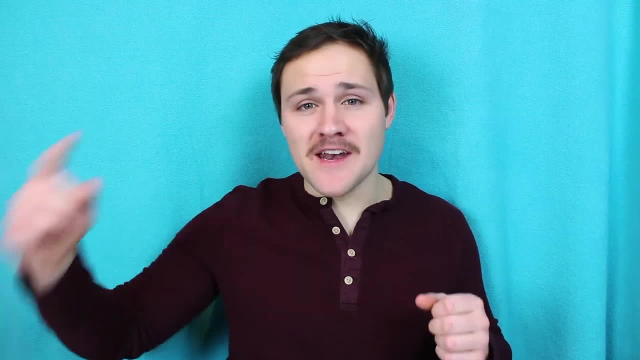 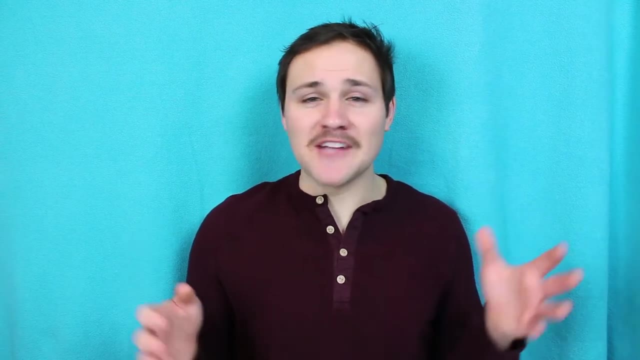 before you finish the rest of the region. If you still can't get them, move on to the next region and come back to those countries. at the very end of the quiz You will get stuck or hung up on certain countries at times. That's just what happens when you're learning every country.